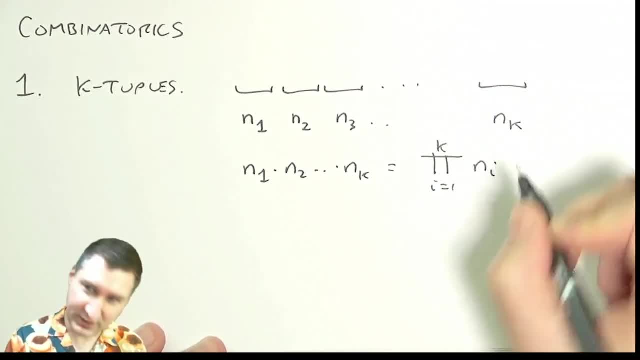 So one way of thinking about this is like with this product notation, where I'm multiplying the number of possibilities for each slot all together, And so, for example, say, I'm in New York State where the license plates have three letters and then four numbers. 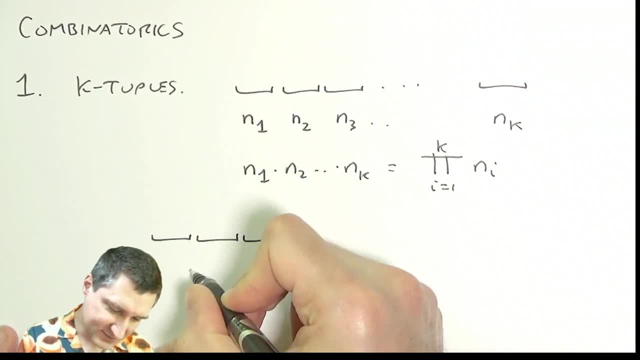 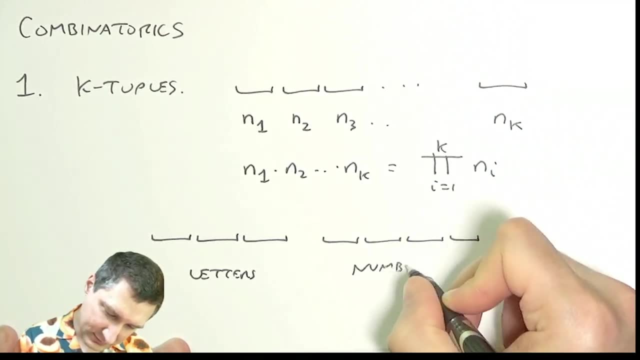 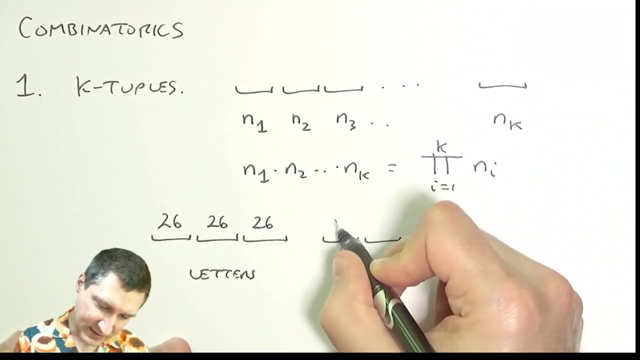 How many possible license plates are there? So I have three slots for letters And four slots for k's, for numbers. so there are 26 possibilities for each of these slots and 10 possibilities for each of these slots, and so the total number of possibilities I have. 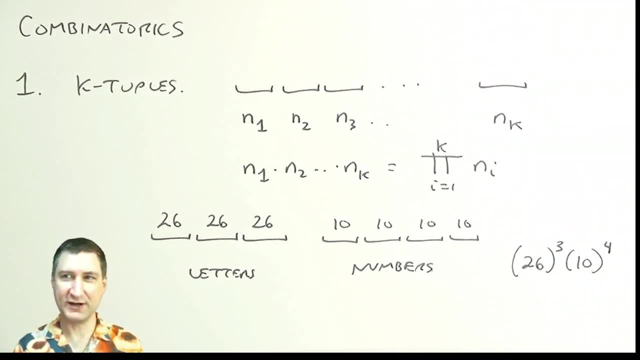 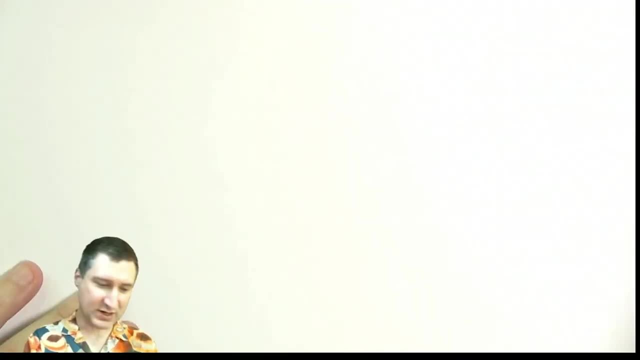 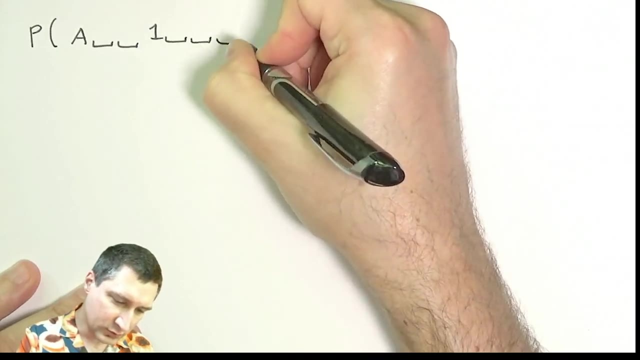 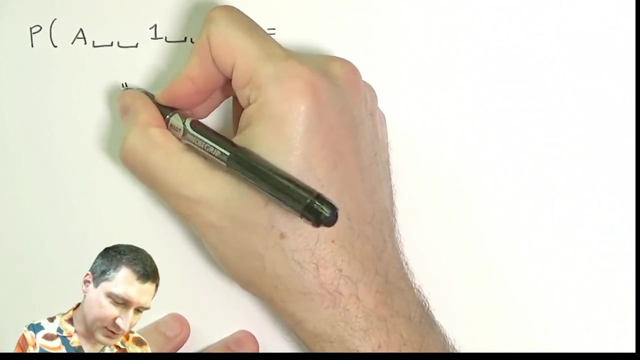 is whatever this very large number turns out to be. And then I can turn this into a probability problem by asking: okay, so what's the probability that a license plate is of the form a blank, blank, one blank, blank, blank? Well, again, I solve this with a counting method. I say: okay, it's the number of. 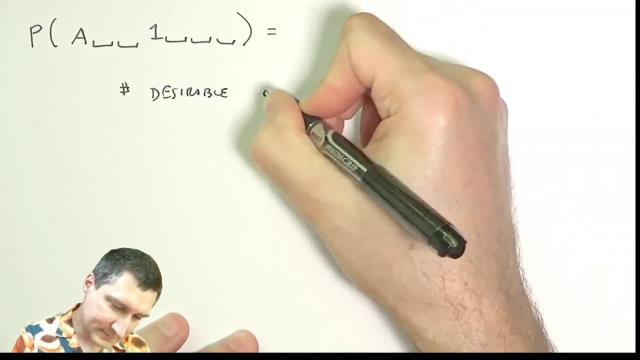 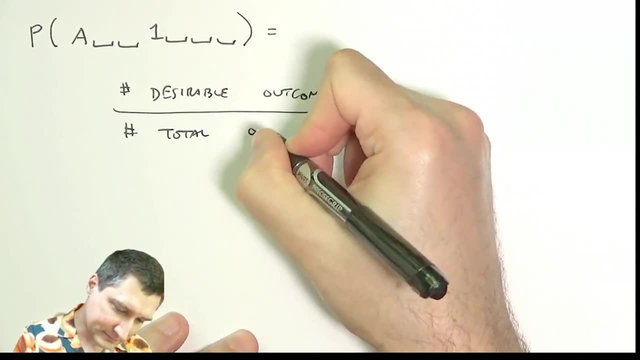 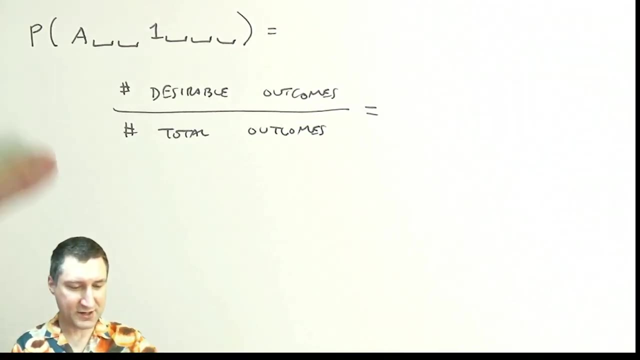 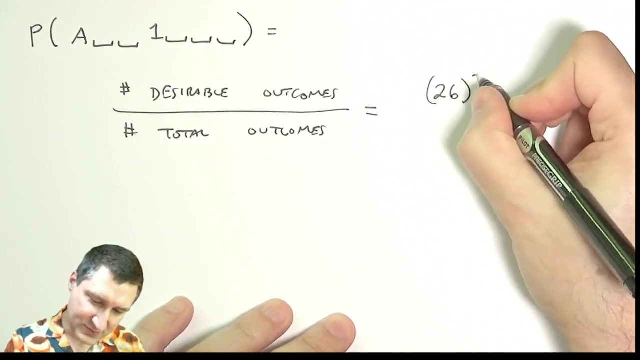 desirable outcomes divided by the number of total outcomes. And so my desirable outcomes are of this form, and here this is like kind of a sub-problem problem Where I say, okay, I have a is fixed, then I have 26 times 26 possibilities for those next two letters. 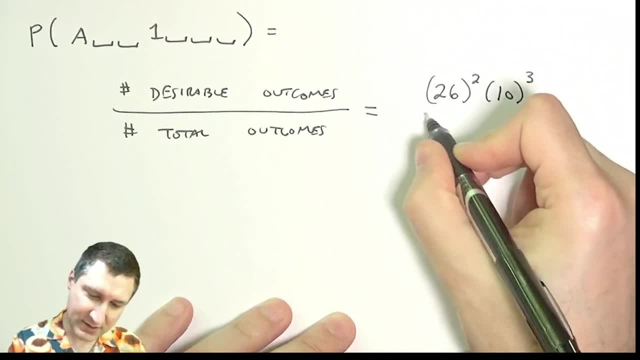 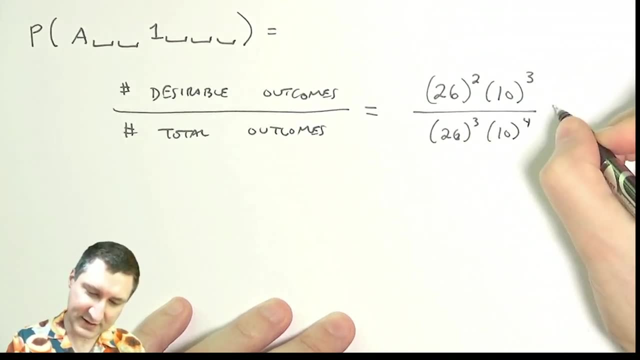 the one is fixed, and then I have 10 times 10 times 10 possibilities for the other ones, and this is divided by the total number of possibilities for license plates that I have, and what's left over is 26 times 10, which is 1 over. 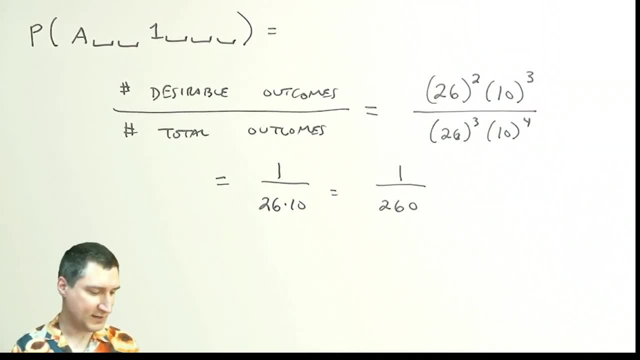 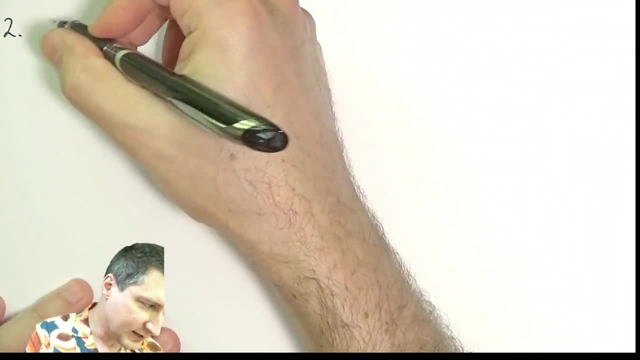 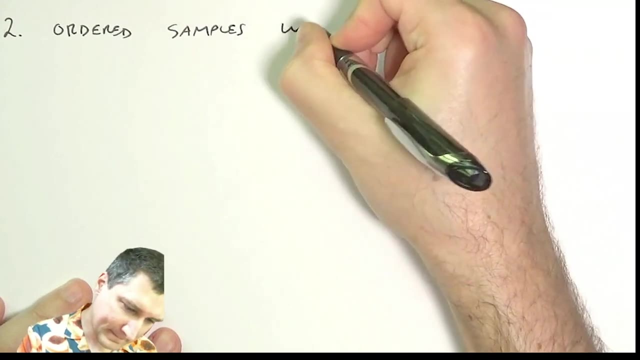 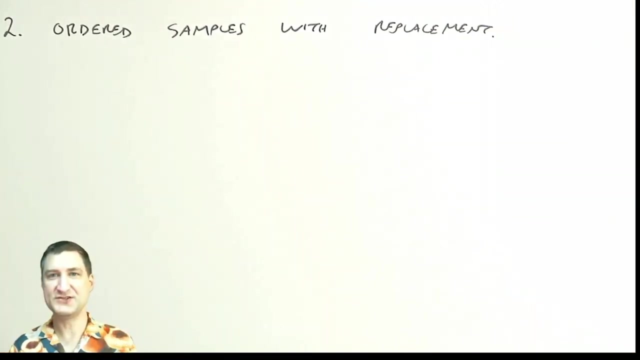 260.. Okay, so my probability of that form is 1 over 260.. Okay, kind of related is to say, okay, what's called ordered samples with replacement. So the situation here is saying, okay, I've got K slots and for every. 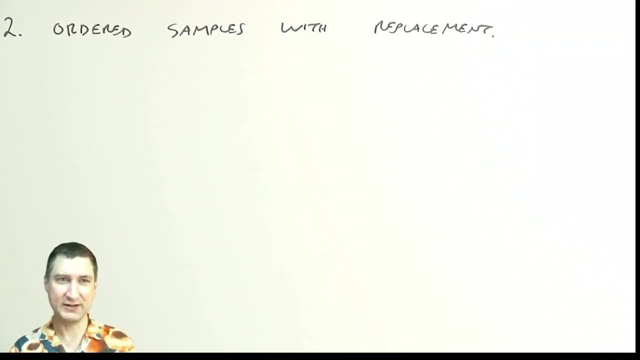 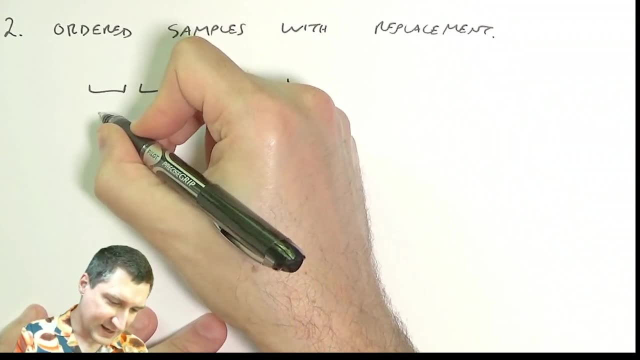 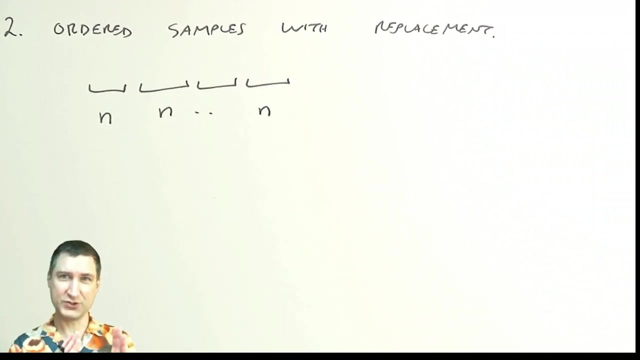 slot I have to put an object in. but after I put the object in I can choose it again. So it's like saying, okay, I have k slots and I have n possibilities for this slot and n possibilities for this slot. So basically it's like saying the previous thing, where my choices per slot is the same for every. 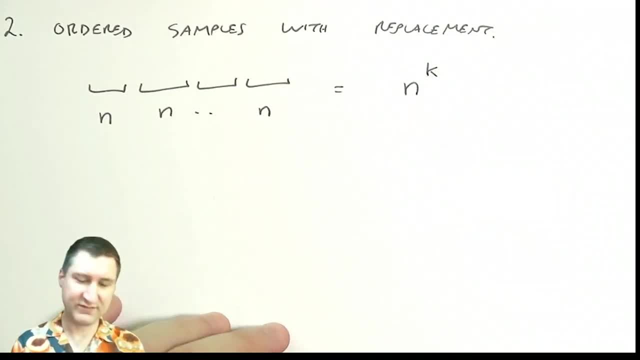 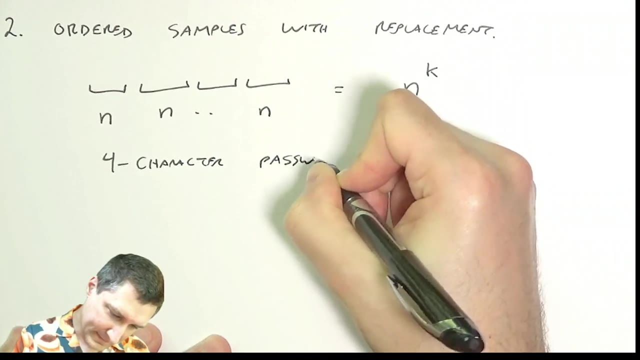 slot. So it's pretty clear that the number of possible sets I have is n to the k. So, for example, this is like saying: okay, you have to choose a four character password, and so that means that there are 26 possibilities for each slot and there are four slots. 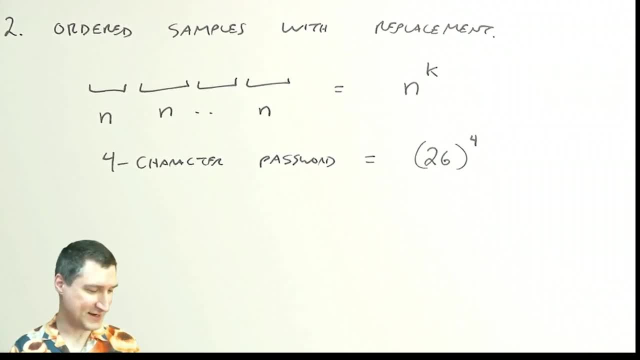 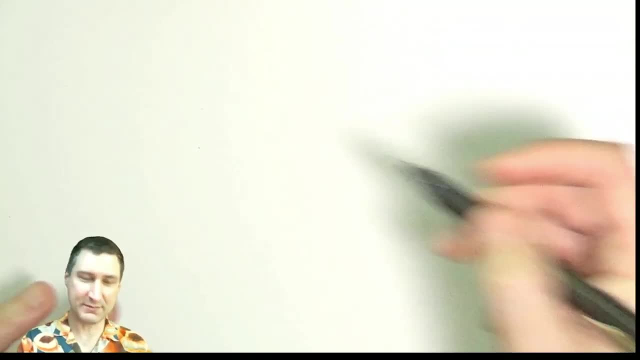 So this is how many possible really easy to break passwords that I have. Of course, in the real world, there are all these constraints on passwords, right? so the next thing that you might put a constraint on is to say, okay, after you choose something, you can't choose it again. So this is called ordered samples. 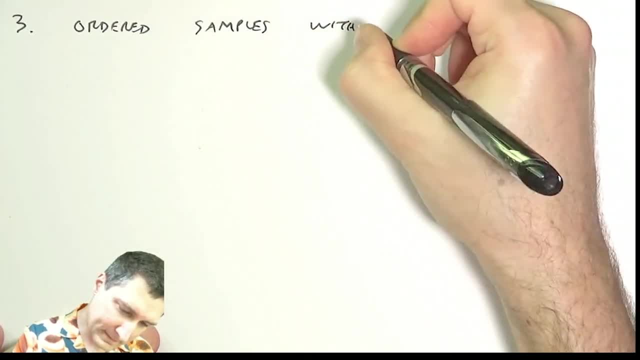 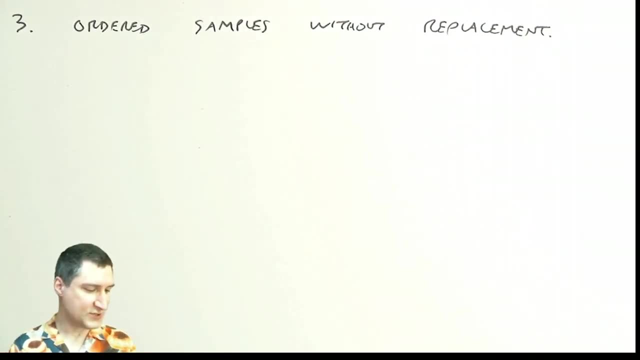 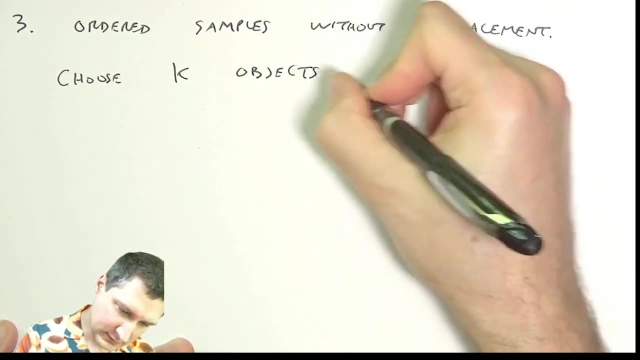 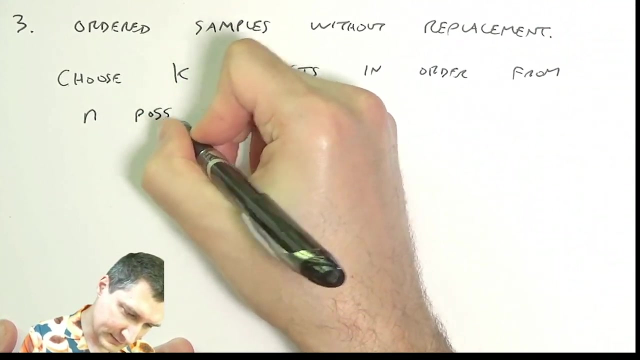 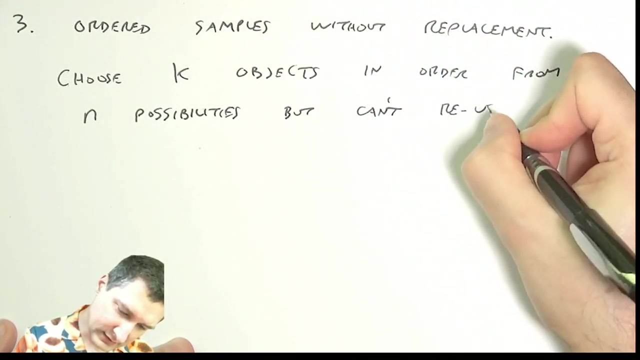 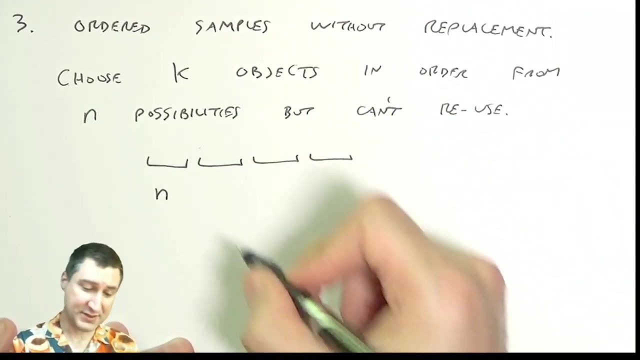 without replacement. So again, I'm choosing k objects in order from n possibilities, but you can't reuse objects. So it's like saying again I have k slots, there are n choices at the first slot, but then there are only n minus one choices at the next. 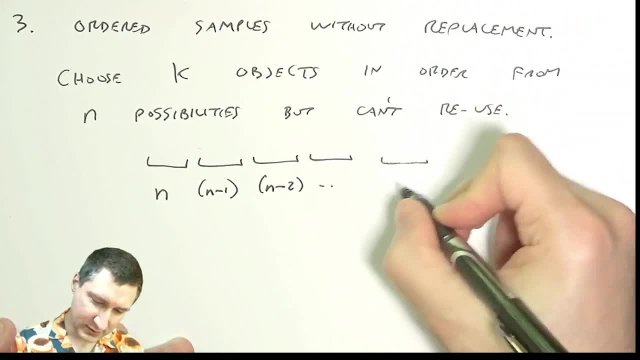 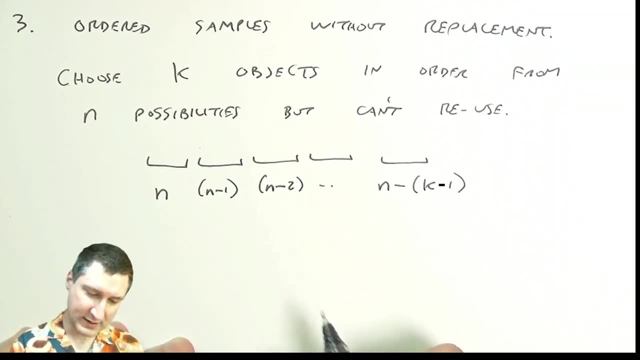 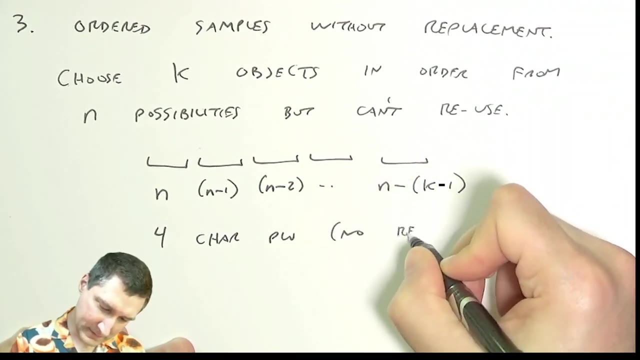 slot n minus two, dot, dot, dot all the way down to n minus k plus one right. So this is like saying, okay, I've got the four character password with no replacement. So that means I have 26 choices for the first 25 choices. 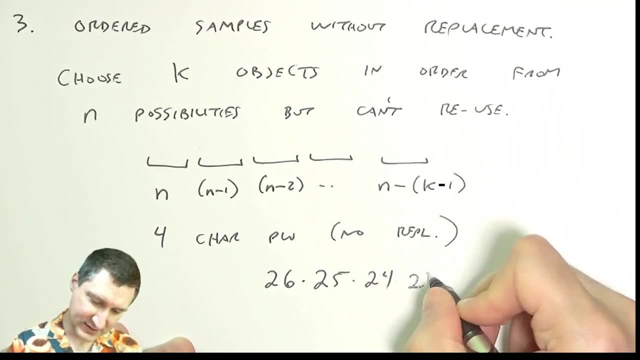 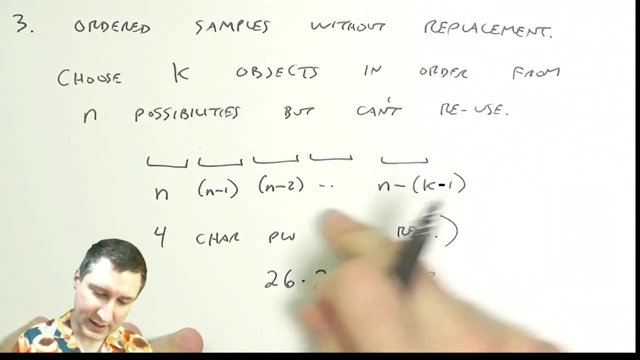 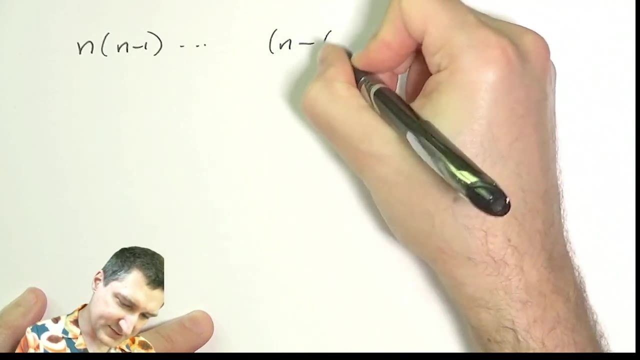 So I have 25 choices for the next letter, then 24, then 23.. So this is actually a smaller number than when I had 26 choices at every slot, right? So this number, which is, you know, n times n minus one, all the way to n minus k plus one, there's a. 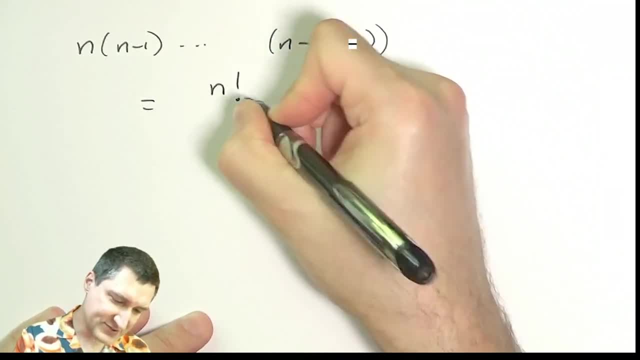 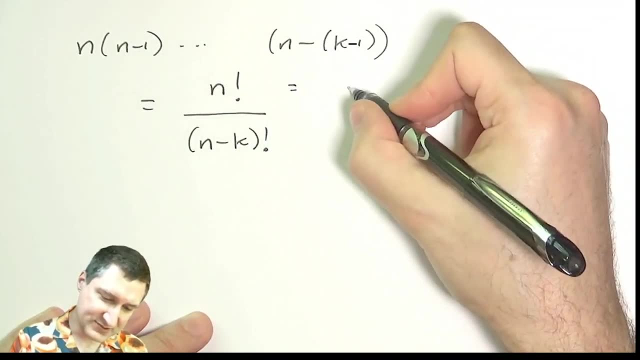 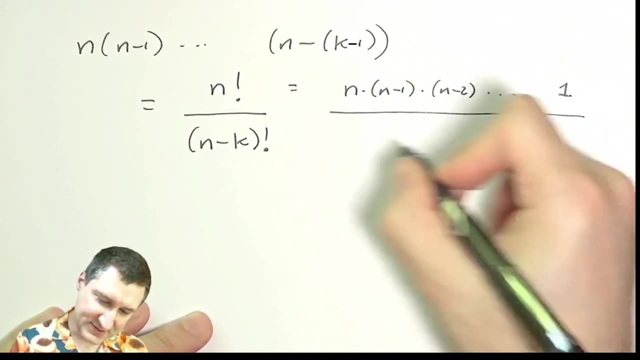 easier way to write this result, and that's by looking at factorial notations. It's like saying: I have n factorial over n minus k factorial, that n factorial is n times n minus 1, times n minus 2, all the way down to 1.. And so that means 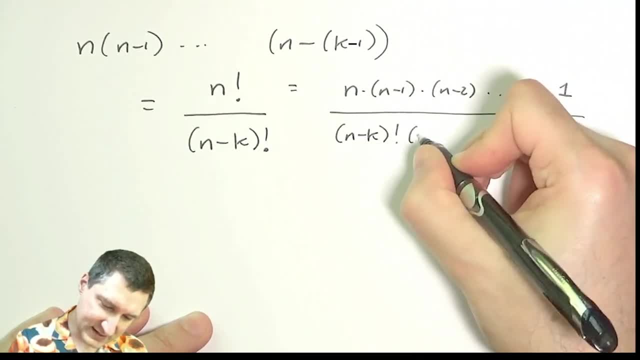 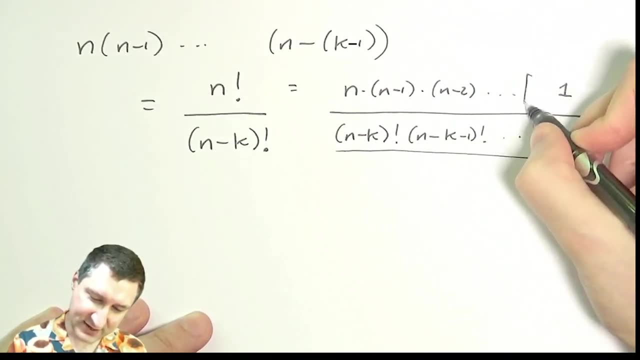 that here n minus k factorial is like n minus k, n minus k minus 1, all the way down to 1.. And so what happens is that this part kind of cancels out all the terms over here, and the last term I see. 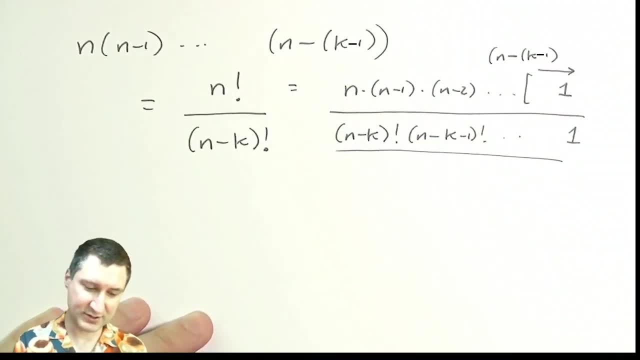 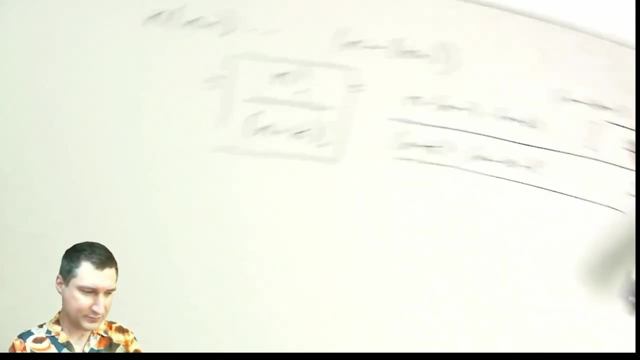 over here is this one, which is exactly this number, right? So this is actually the easier way to write this big number, And usually you know these numbers are kind of hard to deal with when n and k are large. Okay, two more things. Next one is what's called permutations of objects. 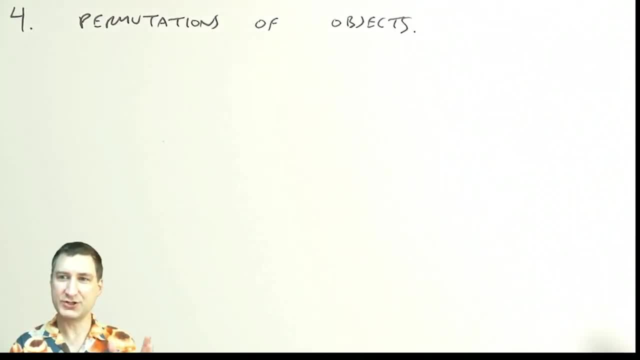 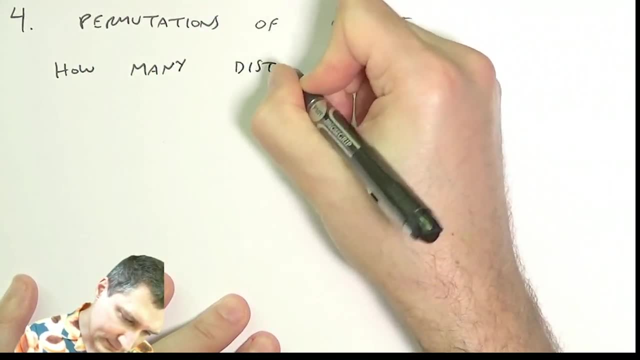 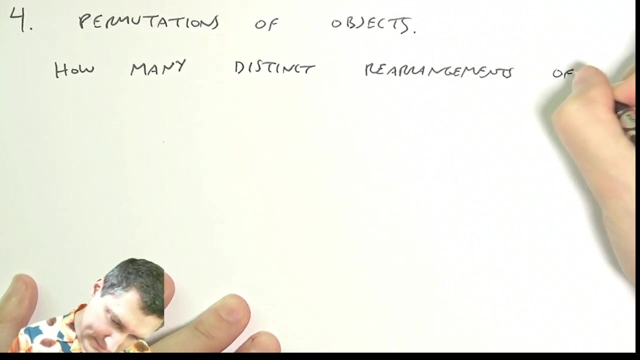 This is like saying: how many distinct ways are there to rearrange n objects, And so actually this is not that different than the previous thing, except it's like saying: I have n objects and I have n slots to put them in. 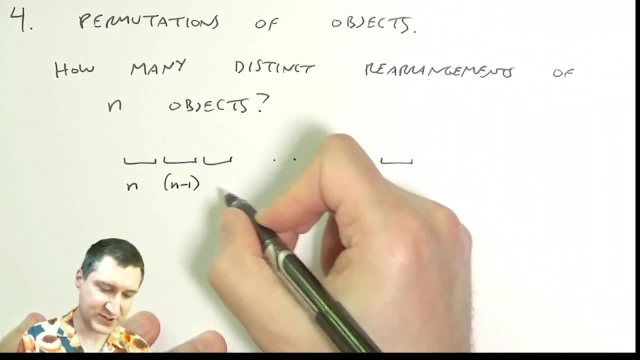 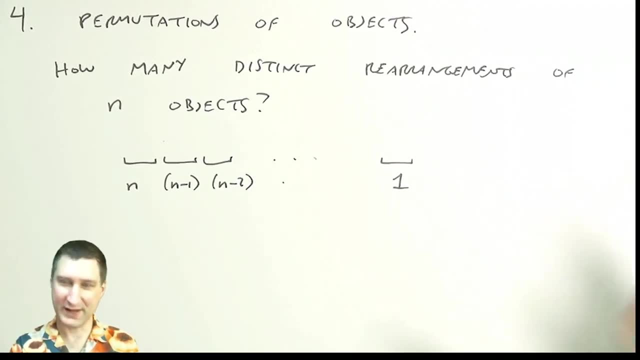 So I have n choices for the first slot: n minus 1. choices for the next one: n minus 2.. By the time I already get down to the last slot. I have n slots to put them in. So all my choices are used up and there's only one thing that I can put in there, right? 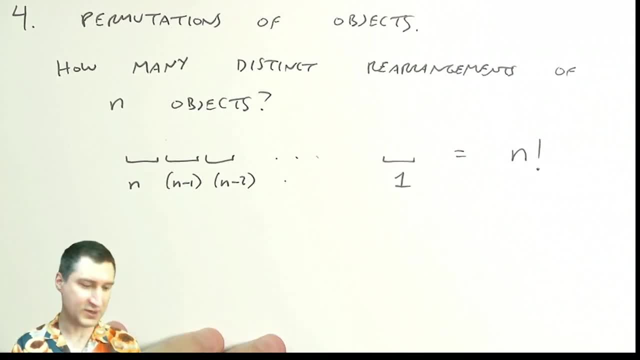 And so this number is actually just n factorial. So there are n factorial distinct permutations of different objects. So for example I could say: okay, you know, a car seats four. This is my crude drawing of a car. And so there are, say: I've got a family of four. 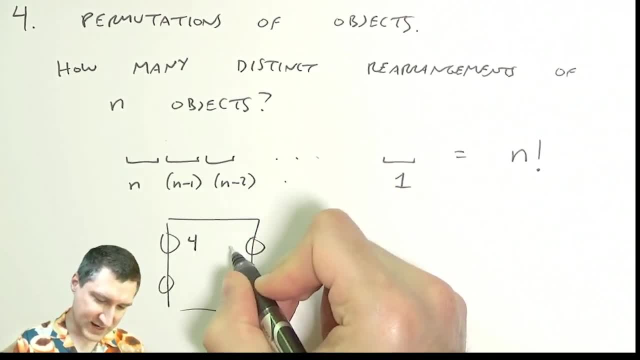 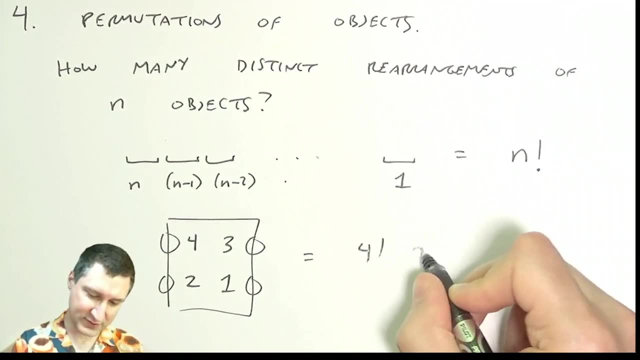 how many ways are there to put those four people in the car? Well, there's four choices for the driver, three choices for the front side passenger, two choices behind the driver and then the person who's left. here is just four factorial, which is 24.. Okay, The last one is what's called 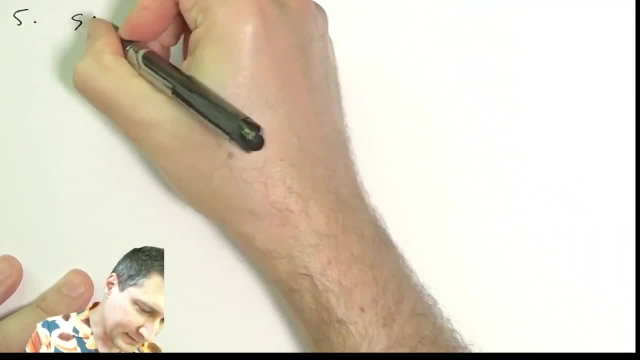 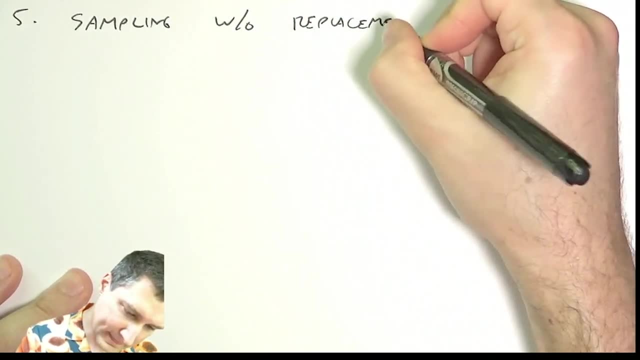 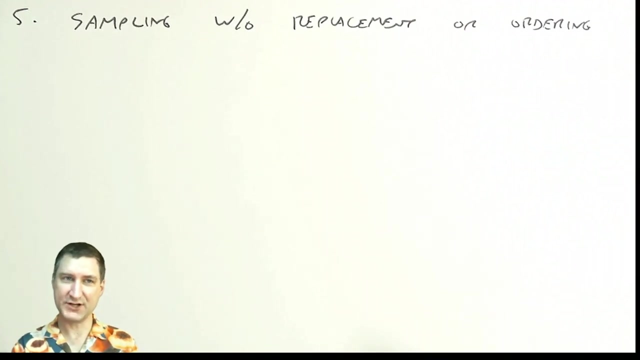 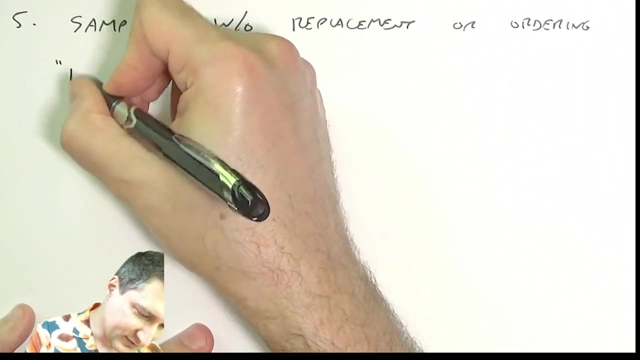 sampling, without replacement or ordering. And this is what happens when we don't care about the order of the objects in the set. we just care about what is contained inside the set. So sometimes you see this phrase in problems like you know how many ways. 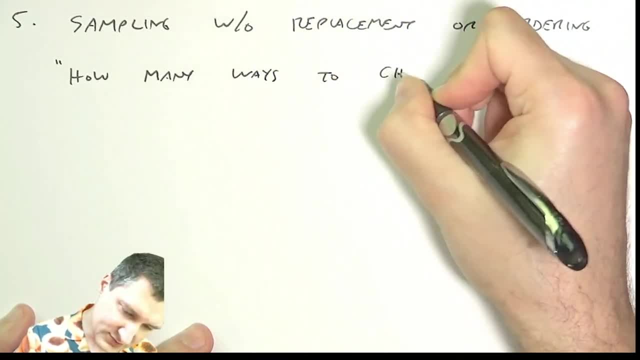 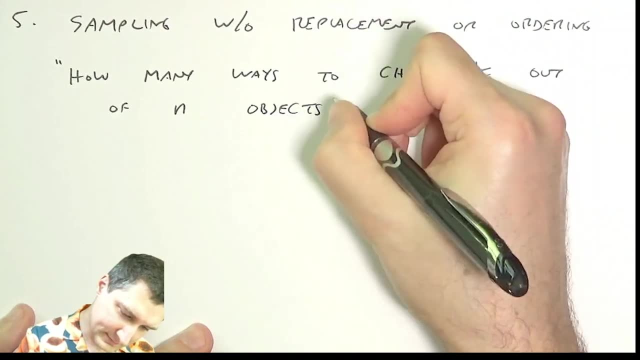 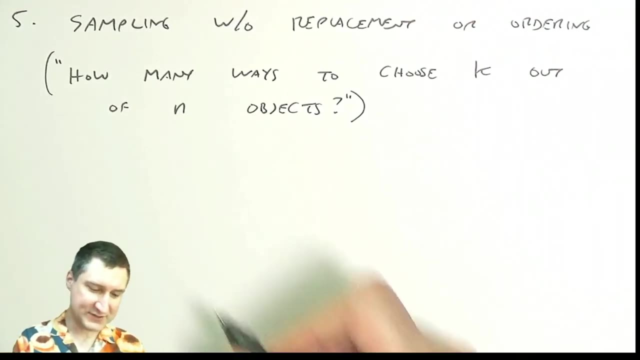 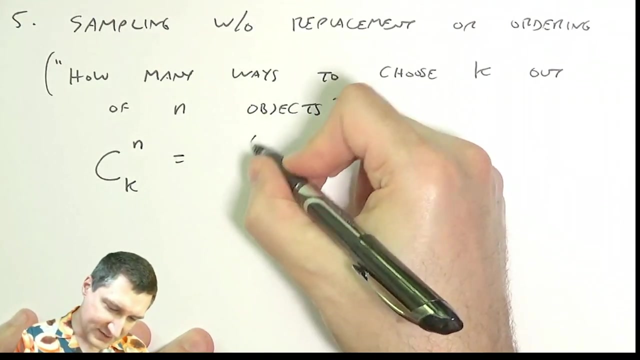 to choose k out of n objects. I guess I should have good notation, And so sometimes you'll see this written like this, with this kind of capital: C with two super subscripts. or you may see it written like this: n, k in this kind of parentheses. 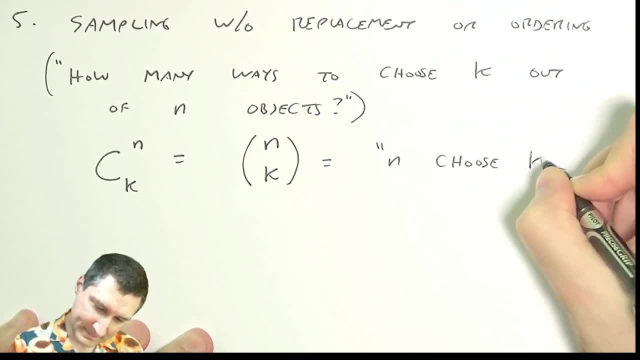 and you may hear it read: n, choose k. Okay, So what is this number? Well, we already know that if I'm going to put, you know I have k slots and I'm going to put choosing n, then n minus one, and so on. that was the previous one. Now I'm like saying okay. 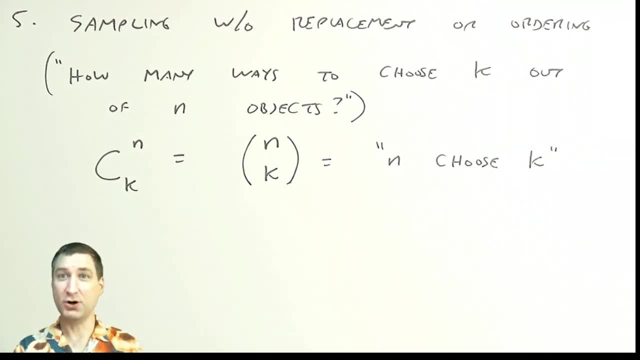 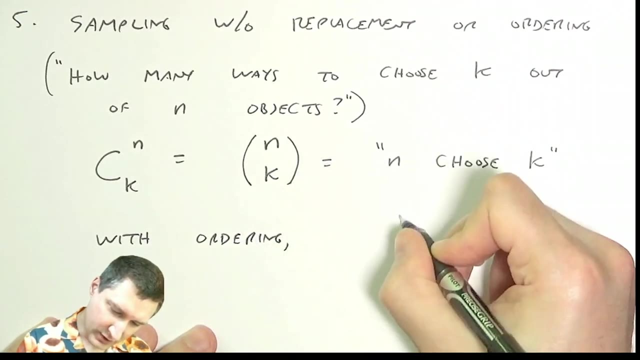 I don't care what the order of these things is, And so that means I've overcounted. if I'm just using the permutation of objects, I have to divide by some number to account for all the kind of doubles or duplicates, right? So with ordering, we already know this is this answer. 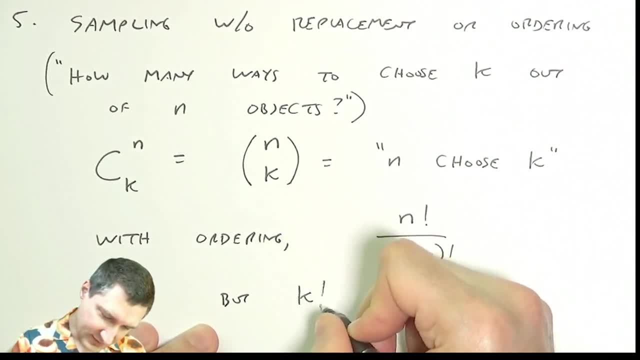 right. But you know, then I say, well, of this set of k objects, there are k factorial ways to rearrange them. So I'm going to put choosing n, n, k in this set of k objects and I'm going to put 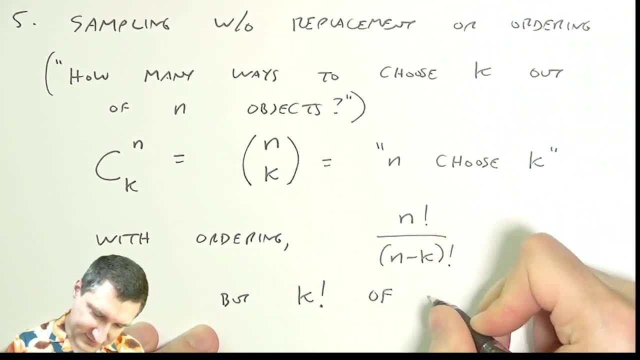 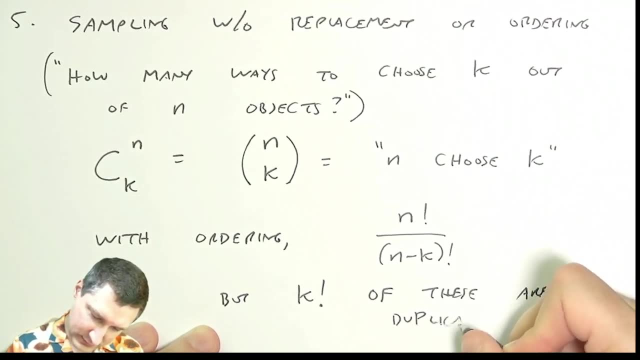 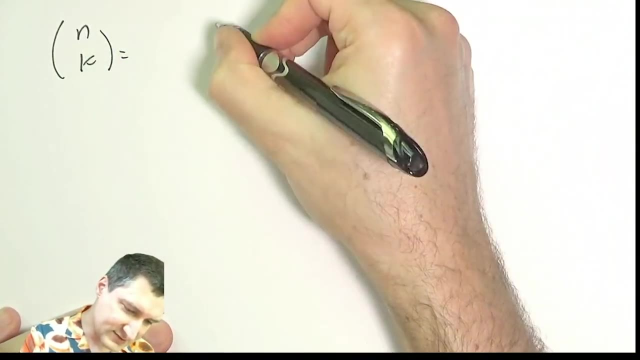 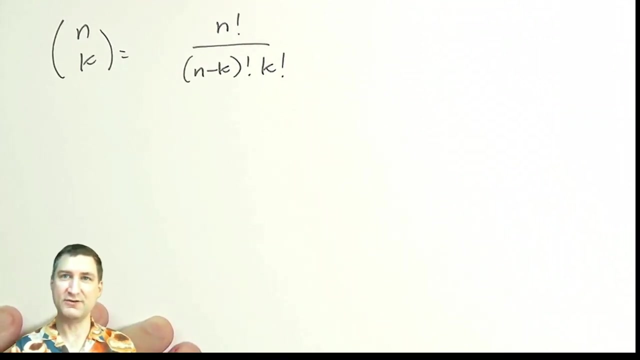 those objects inside the set, So k factorial, these are, you know, effectively the same set. they're duplicates, And so that means that this critical idea of n choose k is n factorial over n minus k factorial, divided again by k factorial to account for all the doubles. Okay And so. 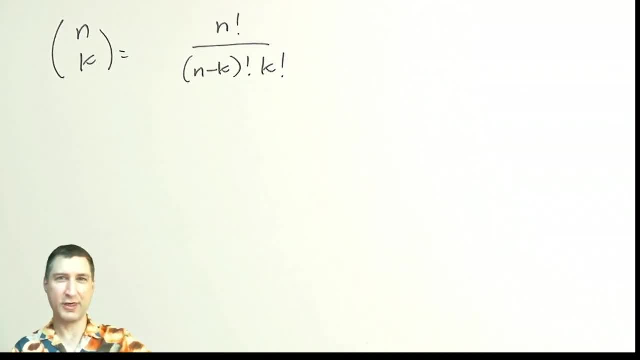 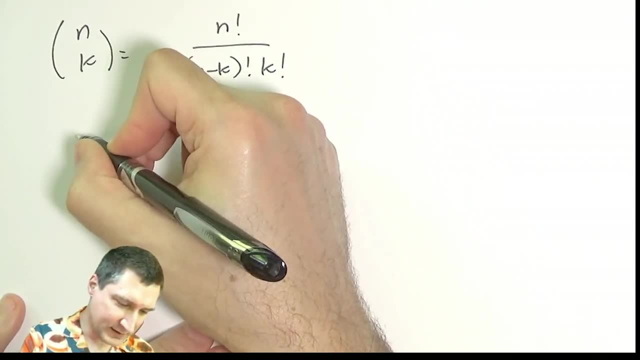 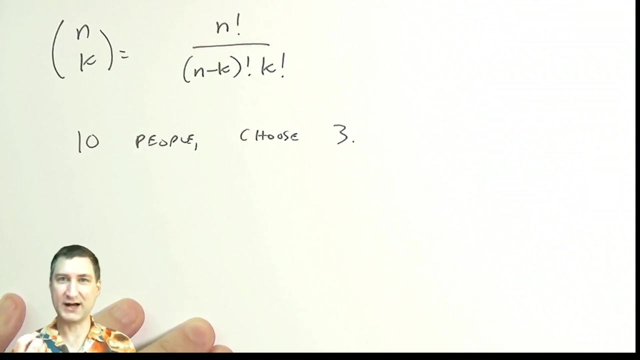 for example, this is like saying, okay, I'm, I'm choosing three people for a team project out of 10.. I don't care what the order that I chose them was in. So I could say: you know, 10 people choose three. How many possible three-person teams? 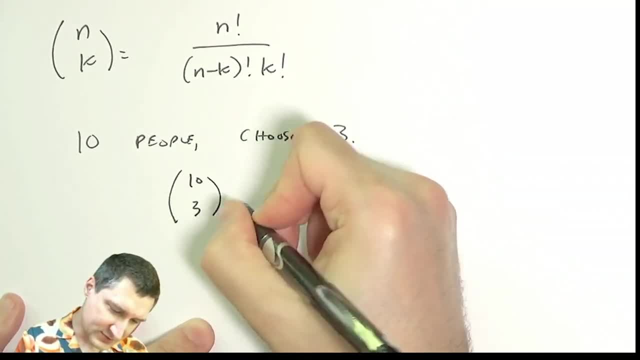 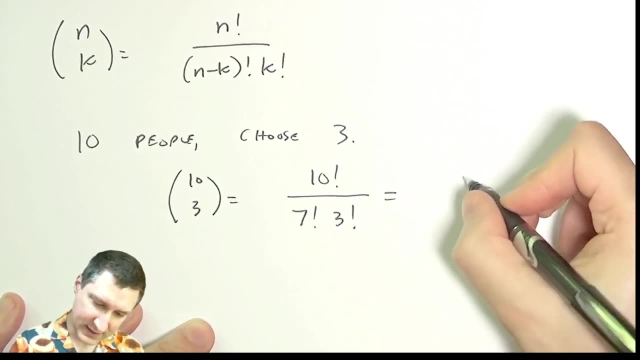 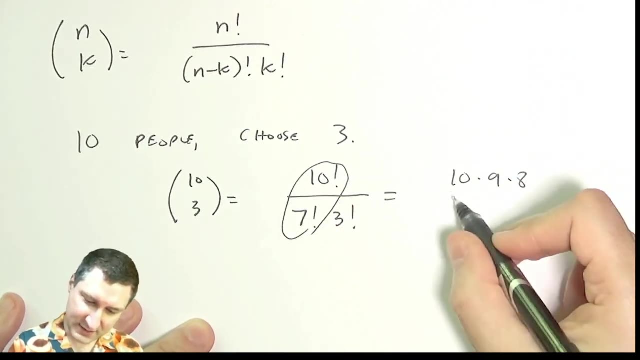 could there be? Well, that's like 10 choose three, which is 10 factorial over 7 factorial, 3 factorial. So if I just were to look at this part by itself, that's like 10 times 9 times 8.. The 3 factorial: 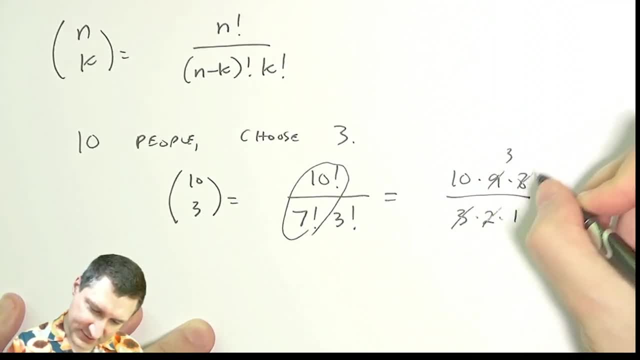 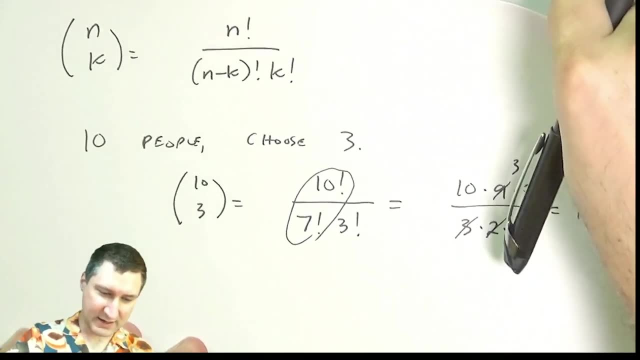 part is 3 times 2 times 1.. And so I can do some cancellations and I can see that there are 120 such possibilities. Okay, A couple other examples. I could say: okay, I've got a ball. 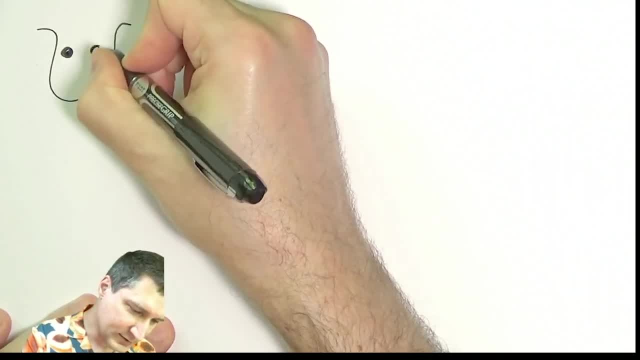 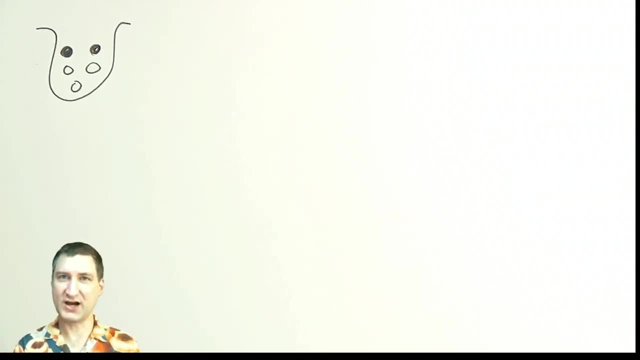 or I've got a bag and the bag contains two black balls and three white balls And I want to know how many distinct permutations are these of of balls, Say, I'm drawing the balls out of the bag and I'm putting them into slots? How many distinct black-white combinations are? 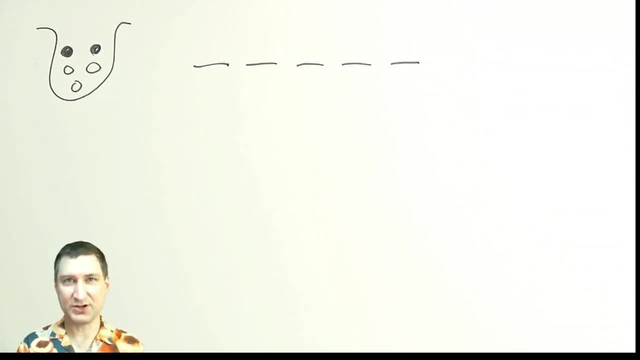 there, Okay. Well, since I can't tell the black balls apart or the white balls apart, there actually aren't that many combinations, And one way I think about this is to say: okay, two of these slots have to be the black balls, right, And so I could think about how many. you know ways. 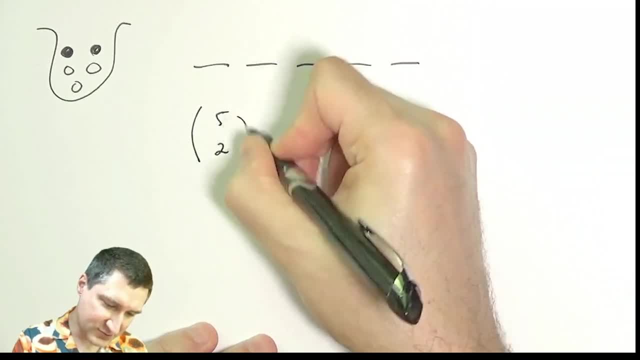 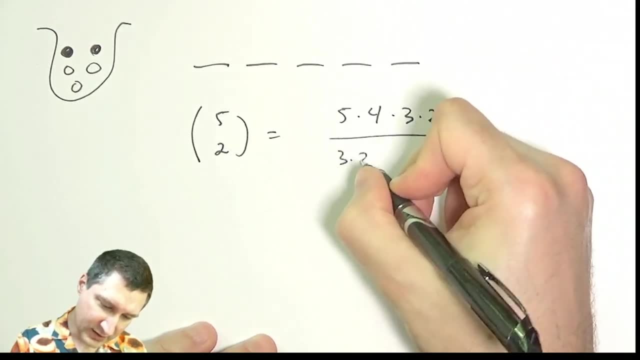 that I could put the black balls in, And so that's just 5 choose 2, which is 5 times 4 times 3 times 2 times 1, over 3 times 2 times 1, 2 times 1.. So I get lots of cancellations And it turns out: 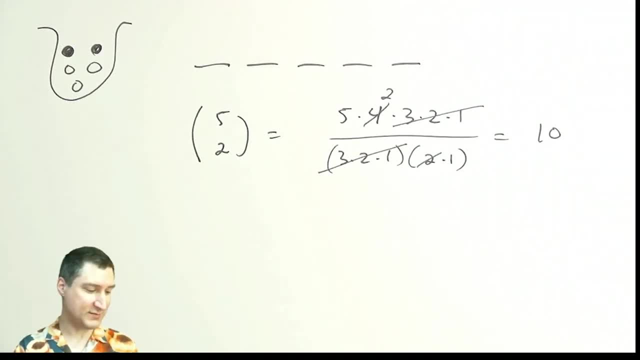 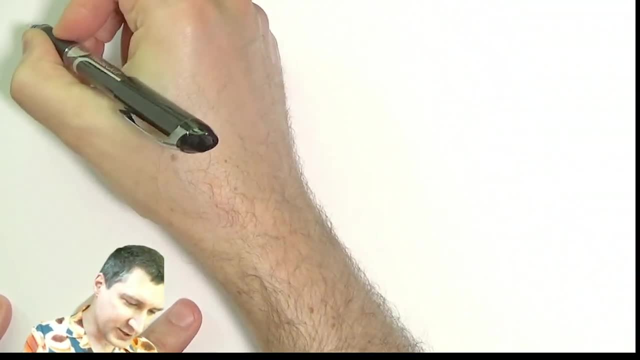 there are only 10 ways of doing this, And if you start to write them down, you can convince yourself that there really aren't that many. Last thing I'll do in this video is: you know a card problem. So let's say: you know a card problem And I'm going to do a card problem And I'm going to do a. 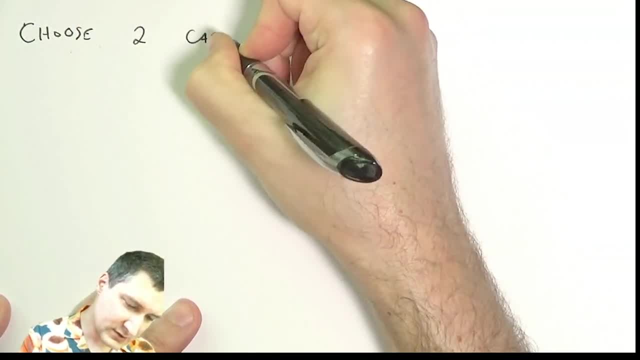 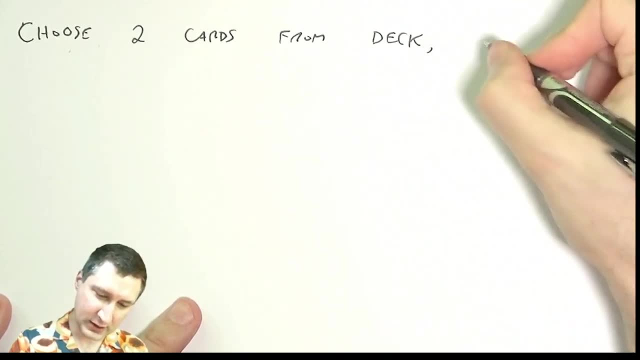 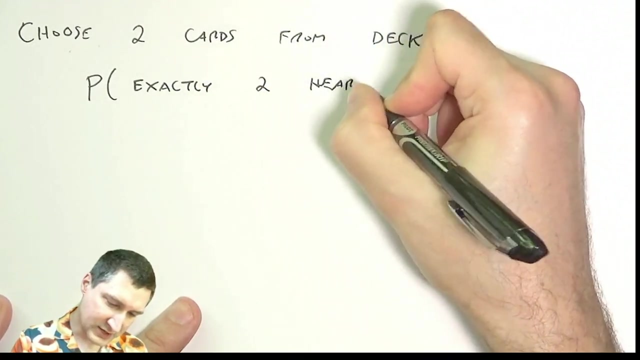 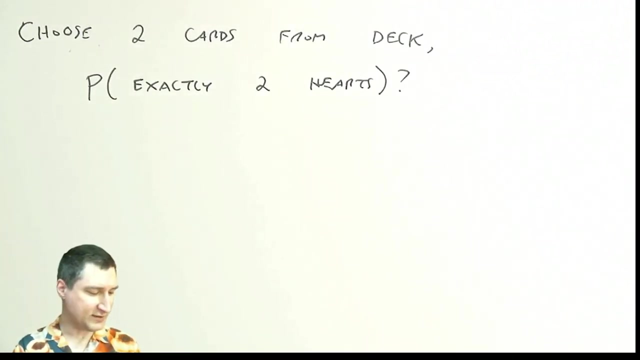 I choose two cards from the deck- normal deck of 52 cards with 13 cards in each suit. What is the probability that I get exactly two hearts, Okay. So again, I don't care about the order of the cards or anything like that. So, same idea, I have the number of desirable outcomes. 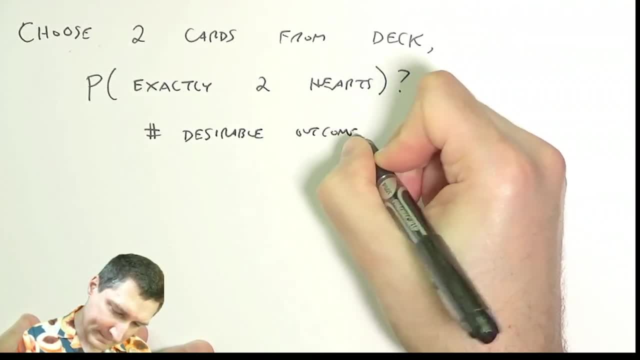 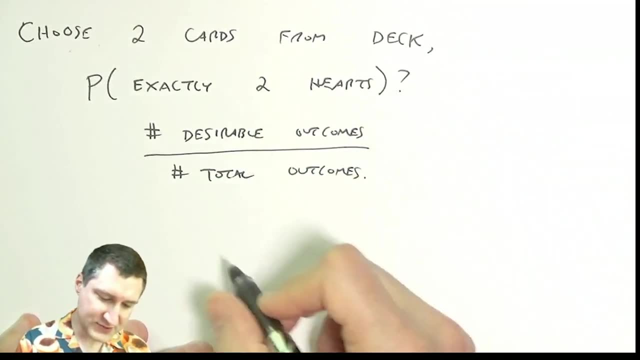 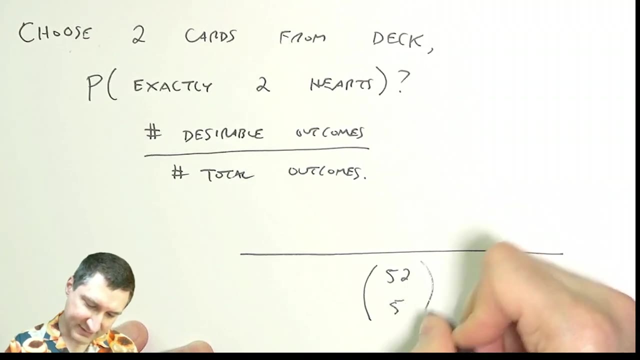 divided by the number of total outcomes. So how many total outcomes are there? Well, there's 52 cards, and I'm choosing 5, right? So that's a big number. And then, how many desirable outcomes are there? Well, it's like saying I need to select exactly 2 hearts.